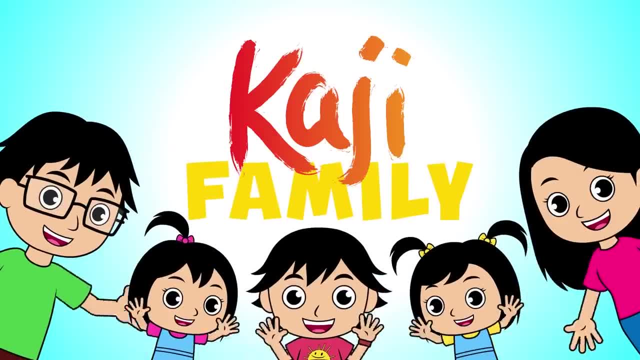 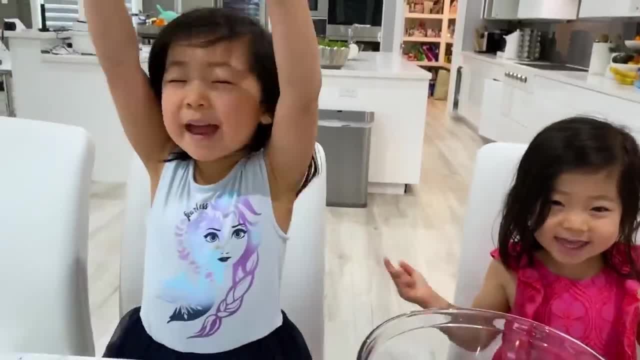 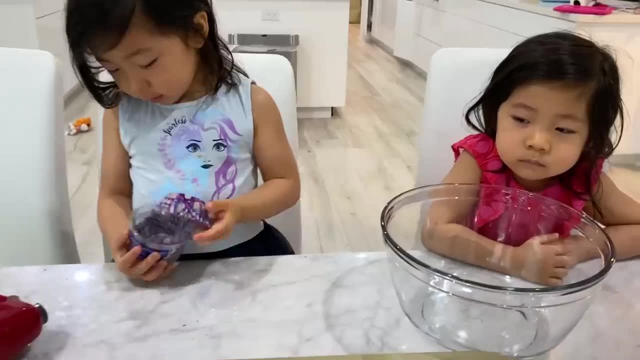 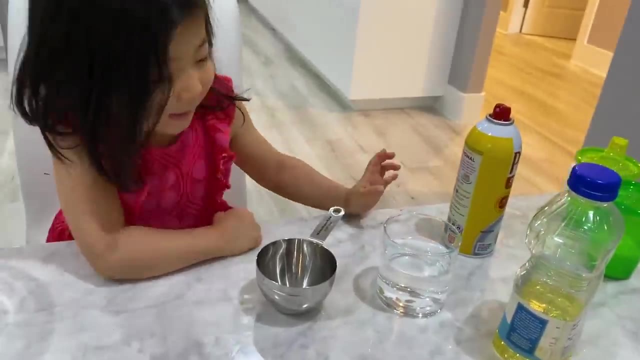 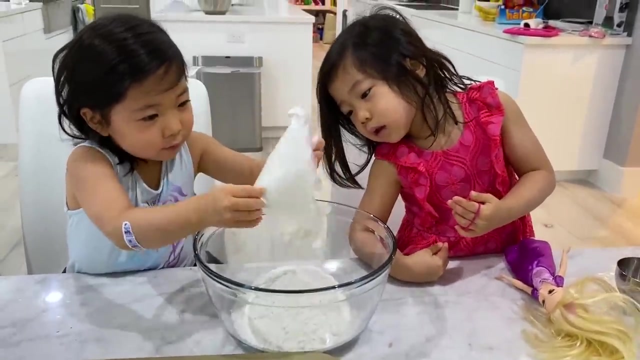 we're making donuts, donuts, yeah. so they really want a big cupcake, and so i just got this um cake mix here, you guys ready? yeah, let's put the whole mix in. there you go. that's a lot, wait, that's a lot. that looks like a casa. 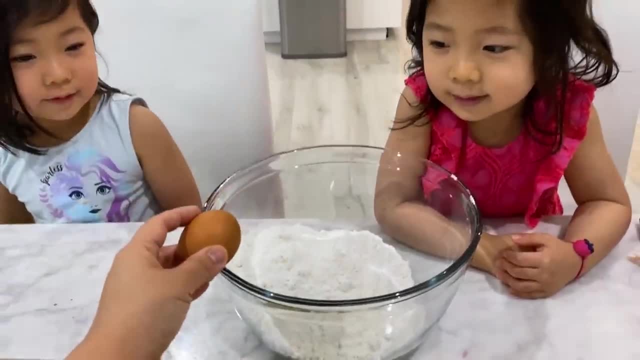 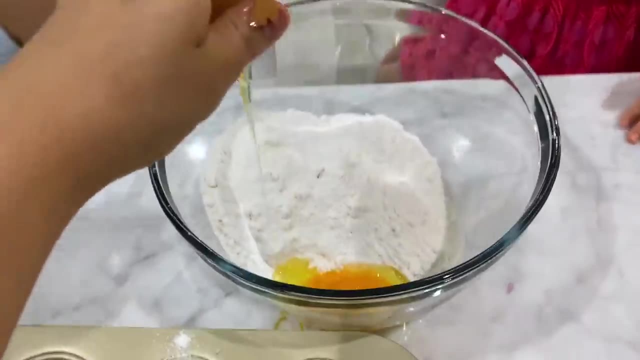 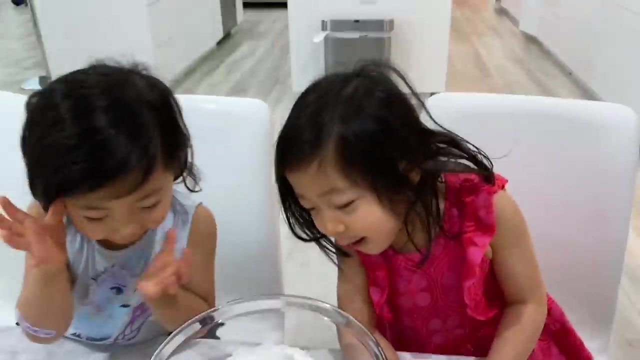 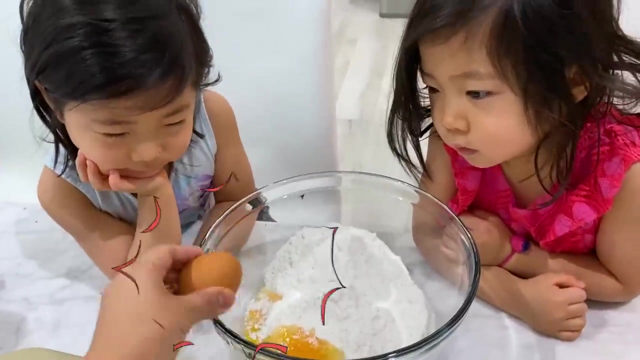 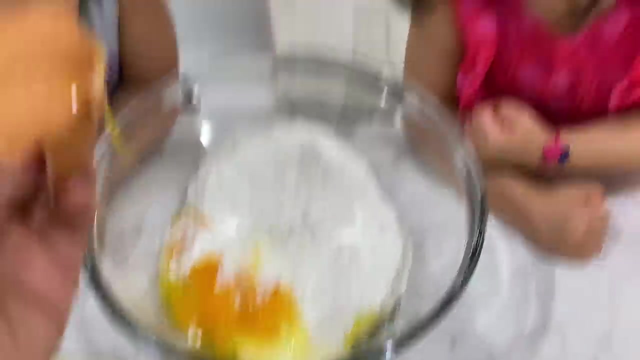 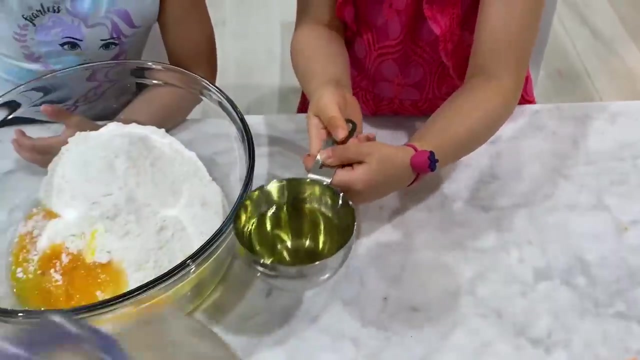 yay, so mommy's gonna do the egg. okay, all right. one, two, three, second egg. wow, do we need one more letter? that's right, one more egg. yeah, last egg. whoa looks cool. huh, yeah, that's super cool. all right, here we go oil. all right, put it in. now time to mix it. i got red. 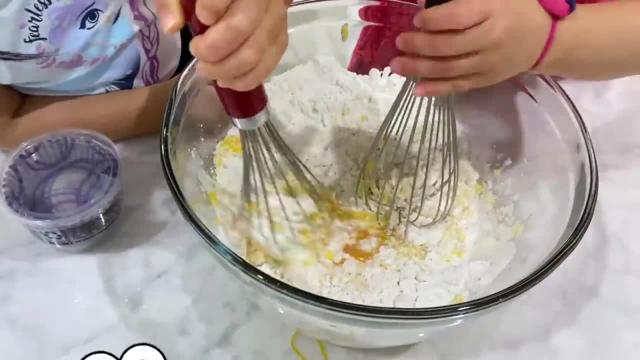 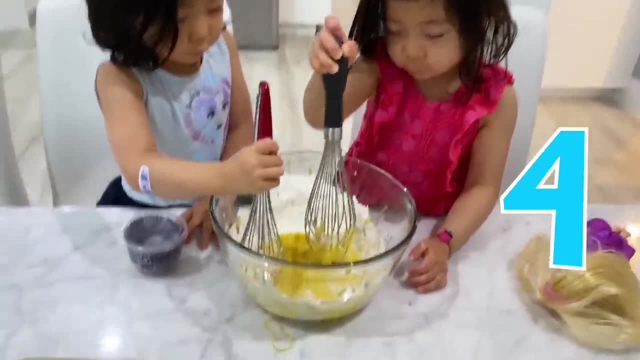 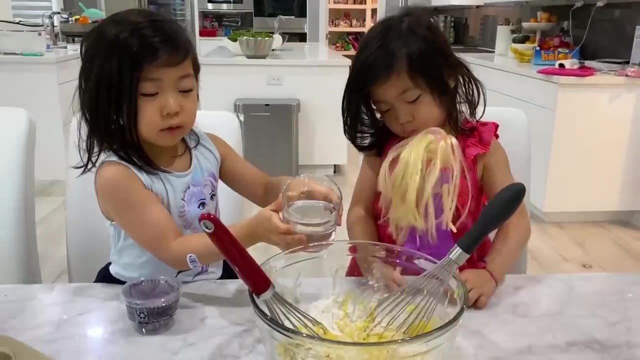 it's inside got me let me put it out. looking good, looking good. everybody mix the cream cake: 1, 2, 3, 4, 5, 6,, 7,, 8,, 9, 10.. Good, We actually forgot water, so now we're adding the water in. 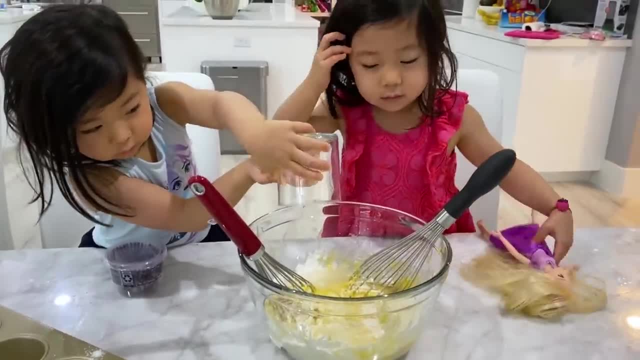 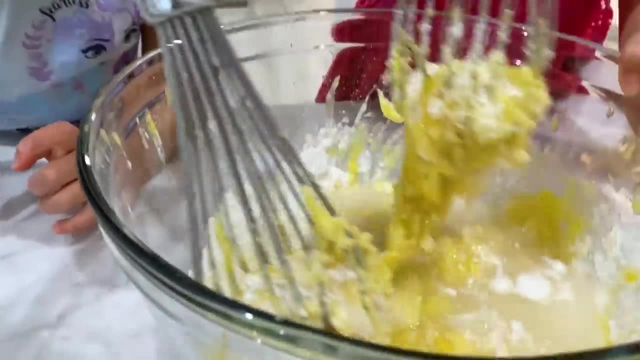 The whole thing. Yeah, the whole thing. Good, Now we need to mix it. Yeah, now we're going to mix it again. You guys are doing good. Whoa, look at the big clump. That looks like water. Yeah, 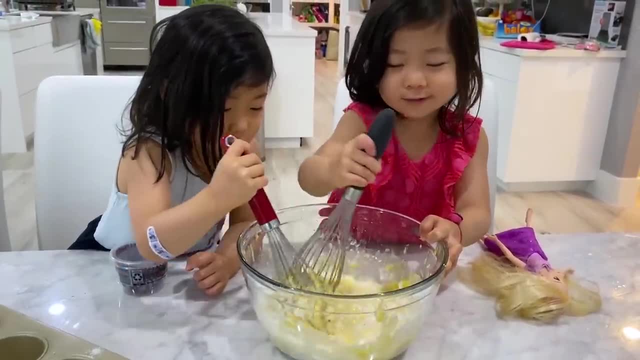 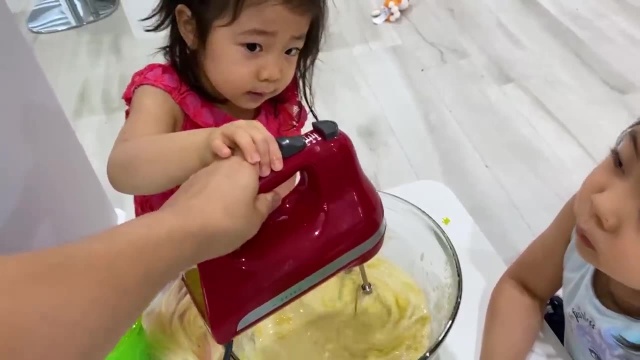 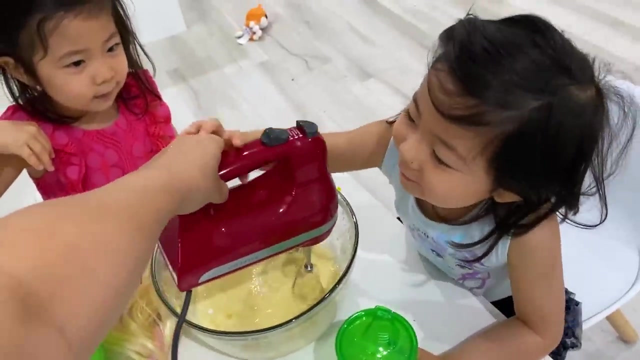 It looks like a pool. It looks like a pool. Yeah, It looks like milk. now It's turning into bubbles, So Emma's going to help me mix. There you go. Good, It's turn, It's turn, Okay. Thank you, Kate. 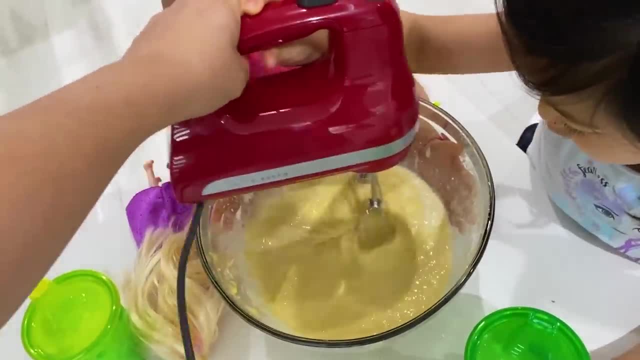 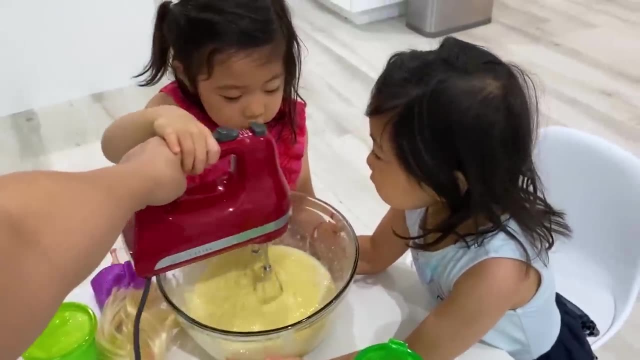 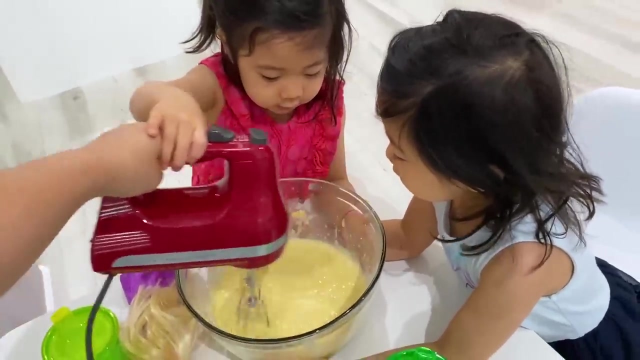 I'm going to hold it. Thank you, Good teamwork. Emma's holding and Kate's mixing. Emma's turn. Aw, you guys are such a good teamwork. There you go. There you go: 1, 2,, 3,, 4,, 5, 6, 7,, 8,, 9, 10.. Good, I'm a dipper, I mix a lot. 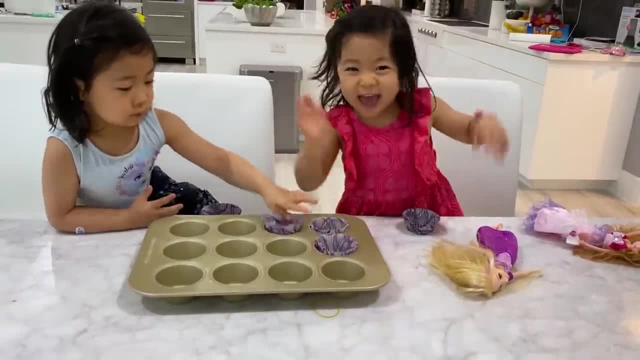 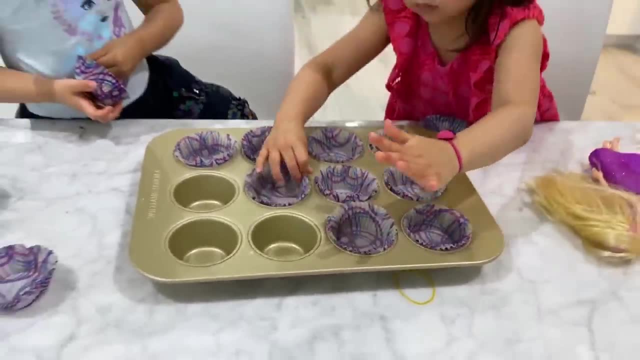 Alright. so next we've got to put in the cupcake paper. There you go, Cupcake. So cool, Good, You guys are doing great. Thank you, Good girls. Let's count to see how many cupcakes we're going to make: 1,, 2.. 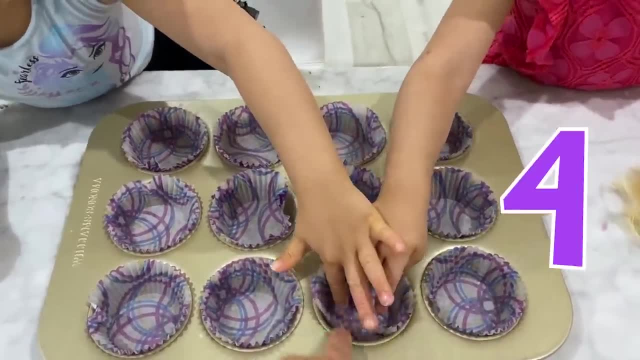 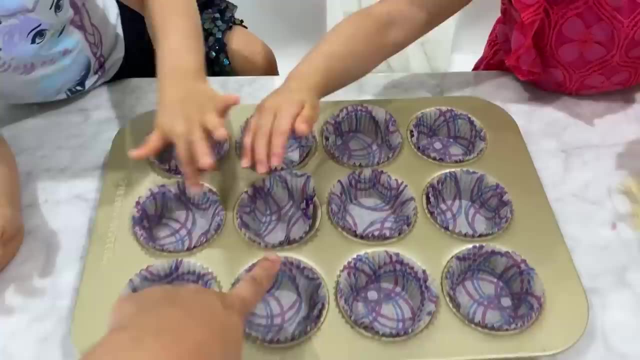 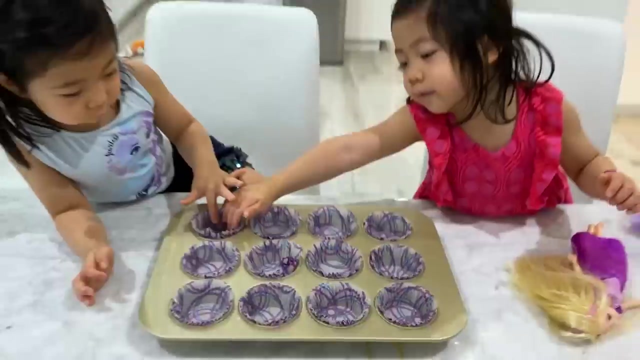 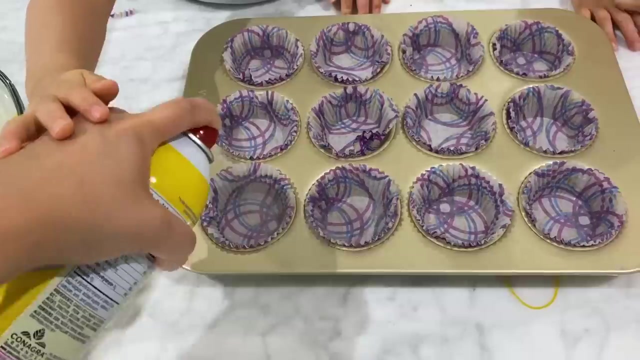 1, 2,, 3,, 4,, 5,, 6,, 7,, 8,, 9,, 10,, 11,, 12.. So how many cupcakes? 12. That's right. The next thing you have to do is spray it, because you don't want it to stick. There you go. 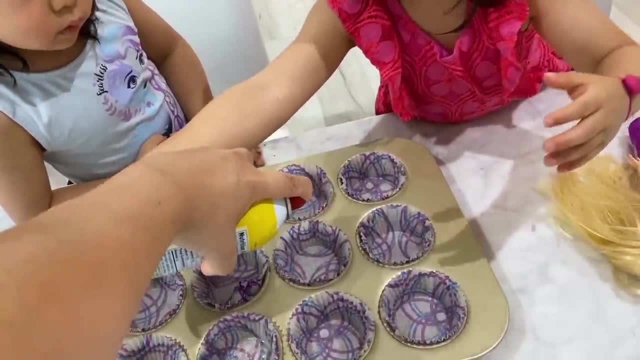 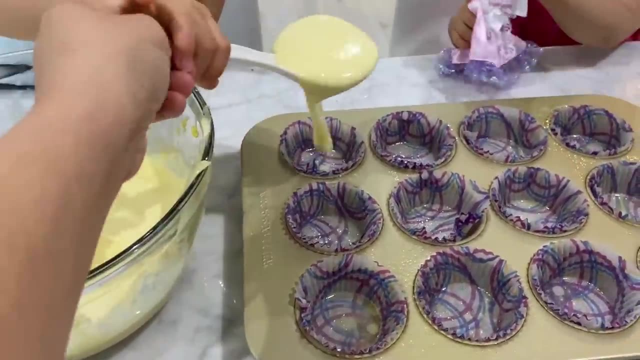 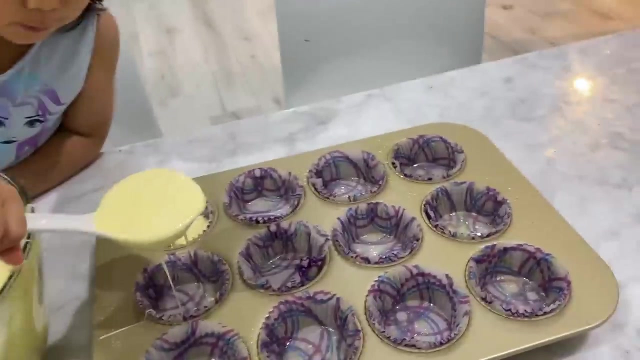 So just spray a little bit. I hold it and you can help me. Okay, Alright, spray it. Okay, perfect, spray, spray. okay. the next step is you're gonna take the powder and then just add it in there. you go see, just like that, whoa too much, huh. there you go, there you. 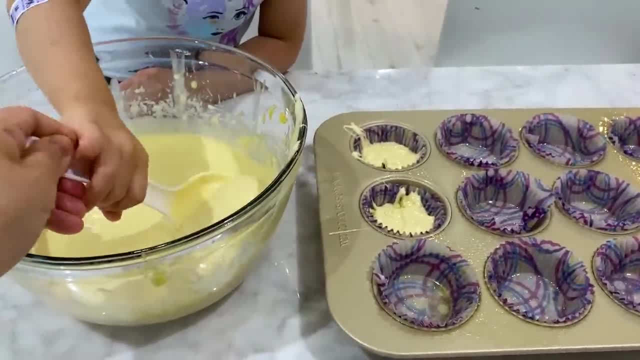 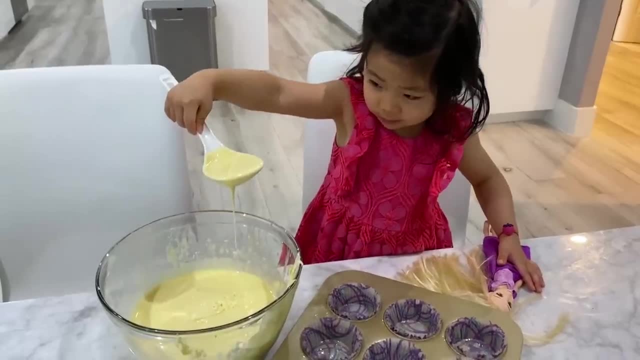 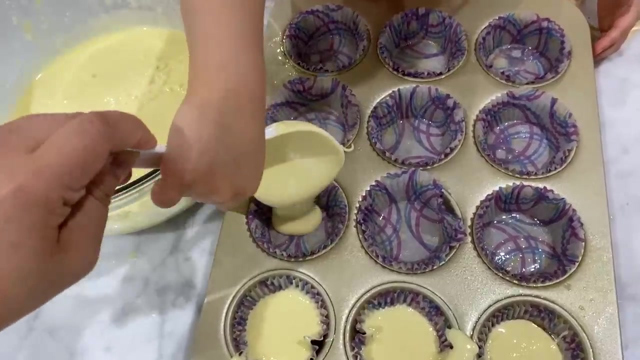 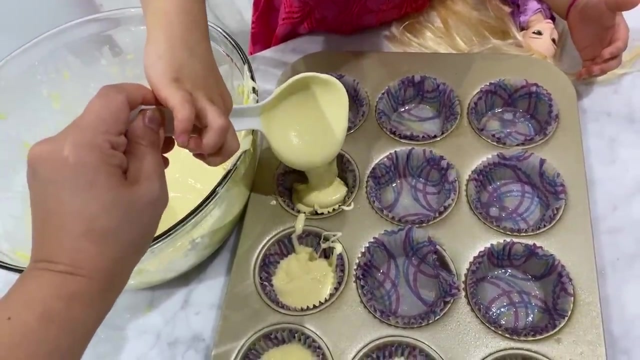 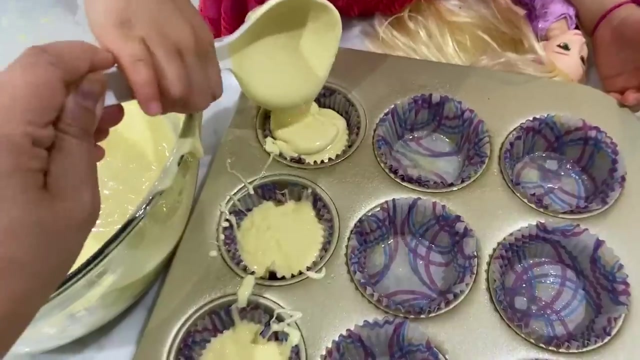 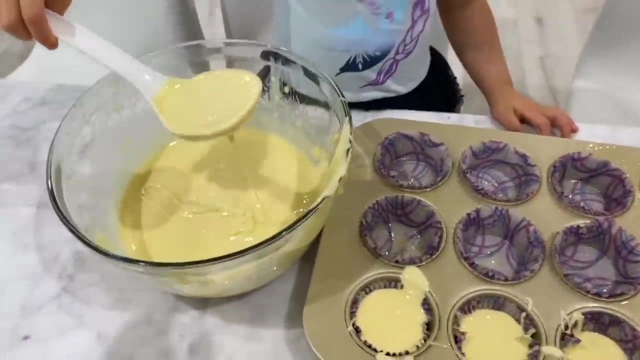 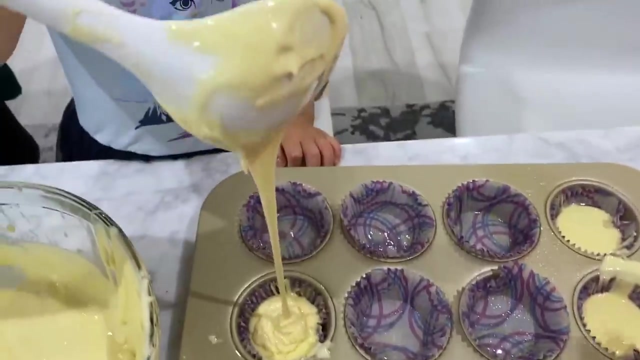 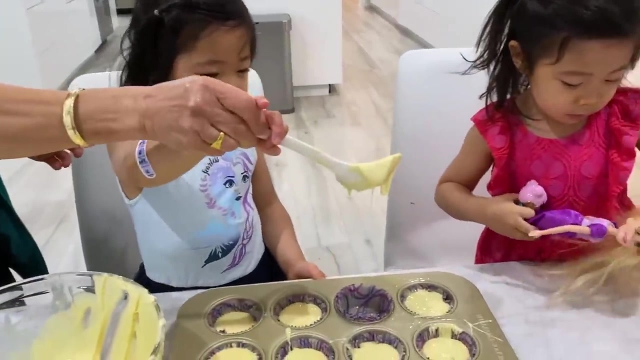 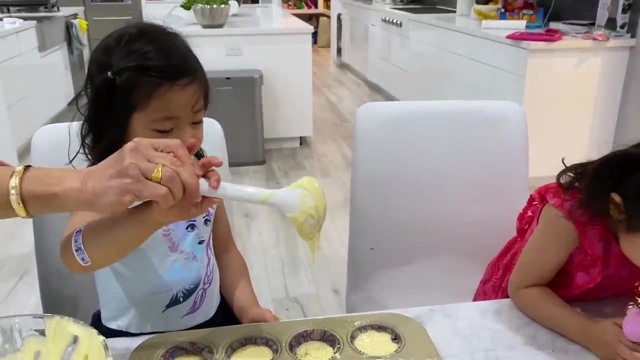 go: nice, okay, that's a big scoop, maybe. okay, there you go. good, girls, yeah, it's okay. okay, now Kate's turn again. yeah, we're learning how to share, so they're taking turns, so we're done with it all. and now you know what we do next. 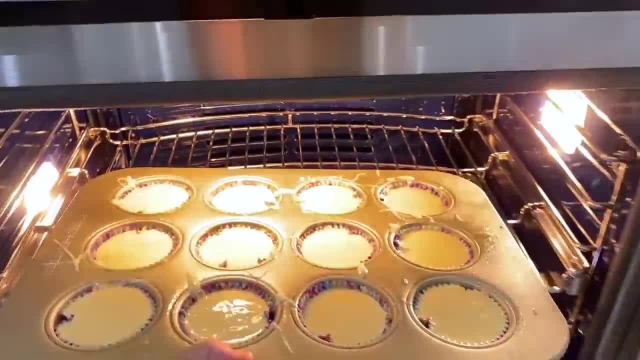 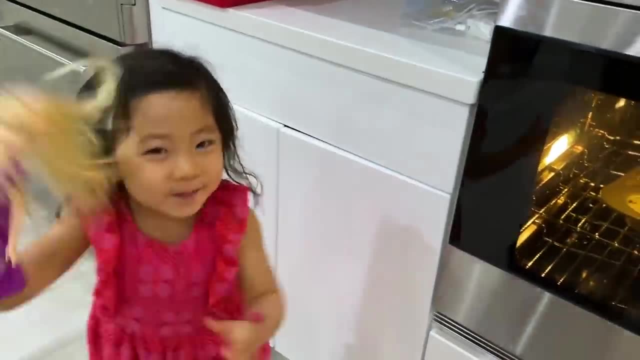 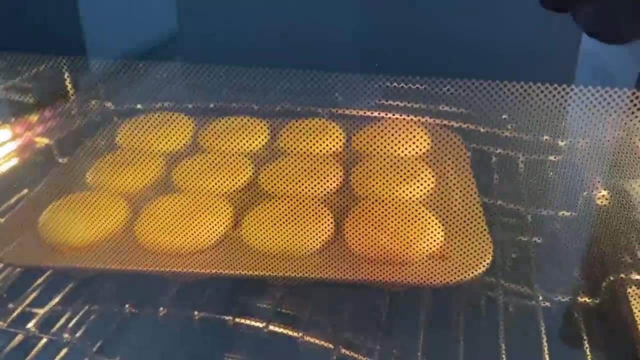 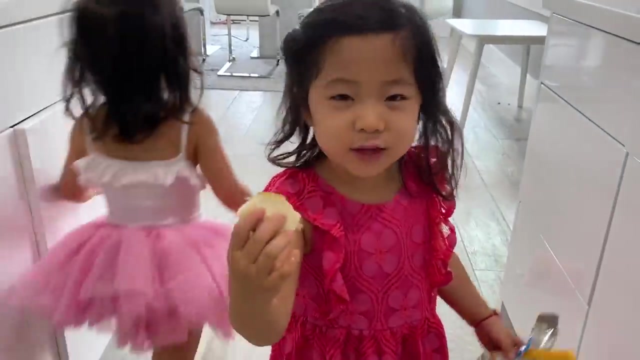 now we're putting the cupcakes in the oven and probably bake it for 15 minutes. there we go. you guys see it's too big, so I think we put too much. look it's too big right now. all right, so cupcakes are done. look how big they become. hi, what you eating there sandwich? yeah, so they're. 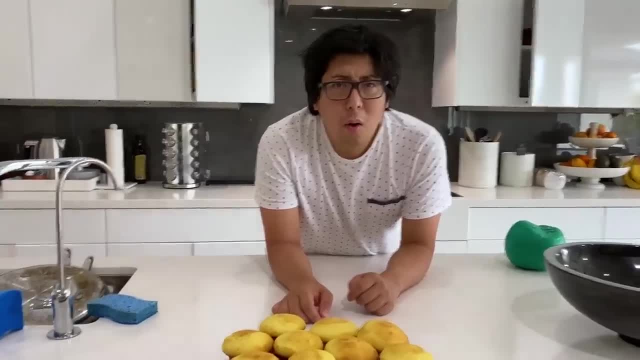 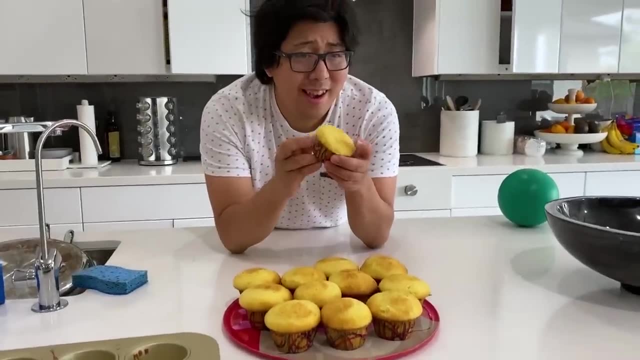 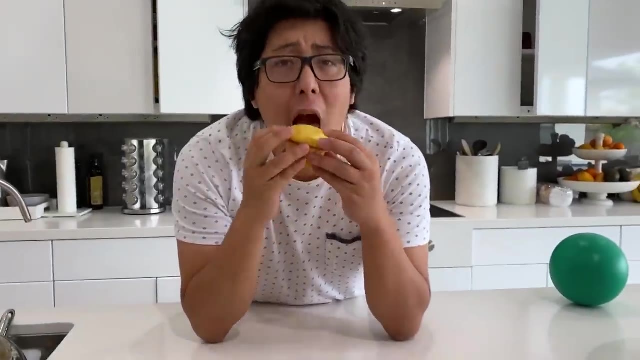 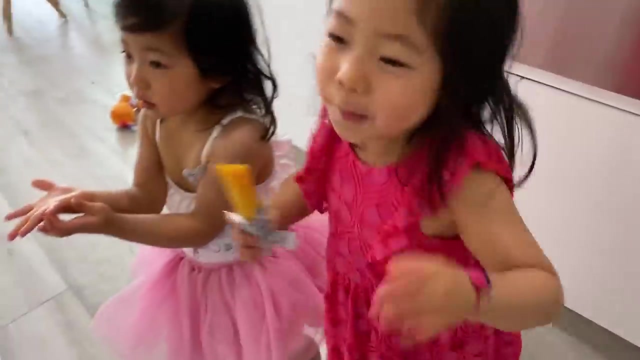 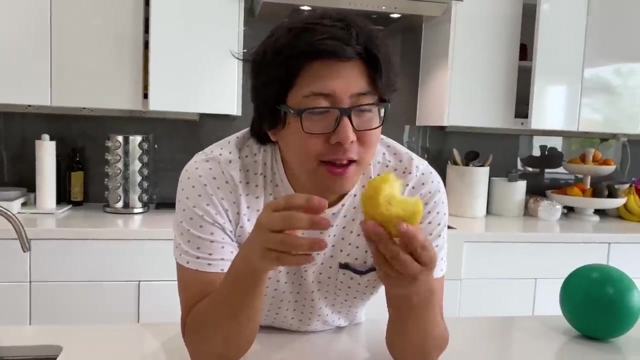 eating while they're waiting for their cupcakes. okay, so daddy's gonna take the first bite. you guys didn't burn it. yeah, we didn't burn it. I like how that's the. is that what you're expecting to happen? I know I was expecting something crispy and hard. 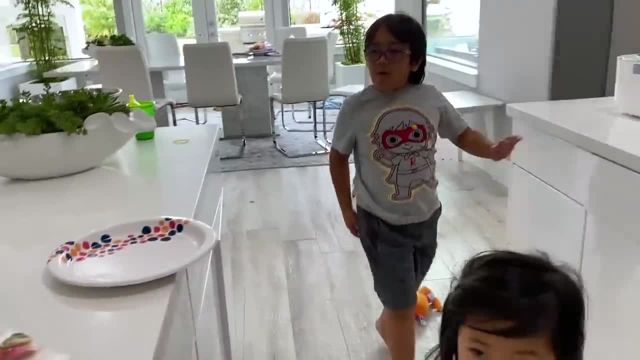 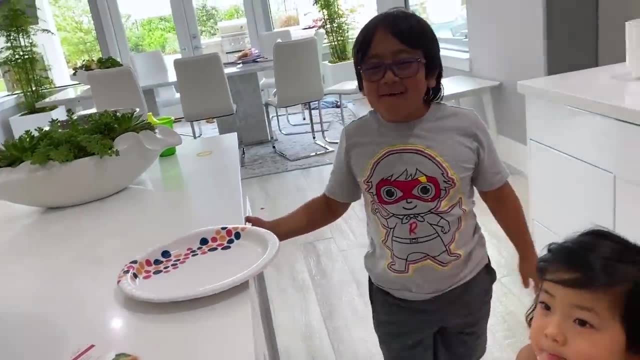 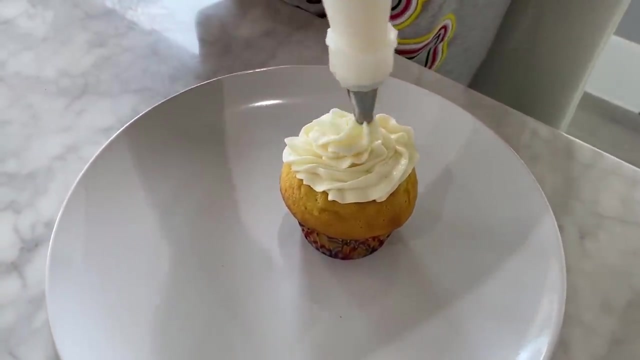 nice and moist, good dog. hey, you want a cupcake, whoa? do you want it with frosting or without? this is without frosting. okay, well, you have to wait. so Ryan's gonna go first decorate his cupcake. there you go. looks good. wow, that's beautiful done. good job, Ryan. and you have some sprinkles. 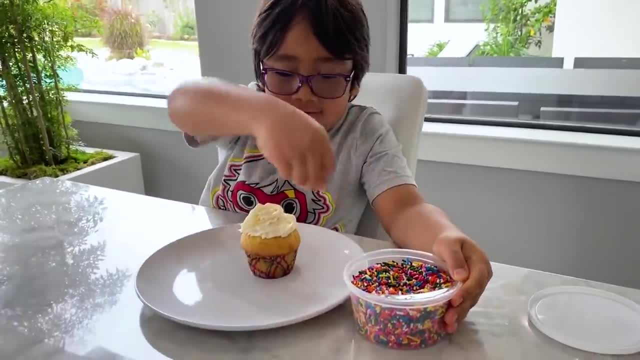 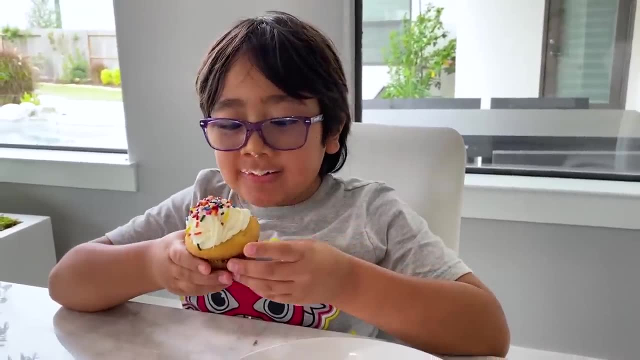 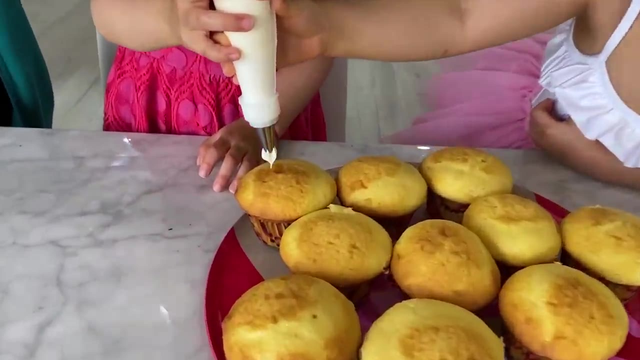 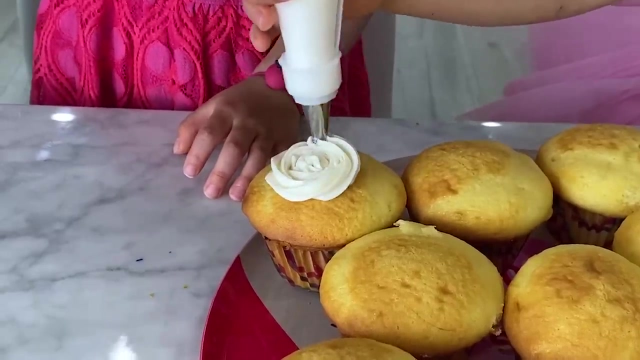 if you want, yeah, let's grab it. yeah, whoa, that's a lot there you go enjoy, yeah, a cupcake stash. so now grandma's gonna help them. there you go. you got a swirl. not too much, yeah, you guys are doing great. not too much okay. 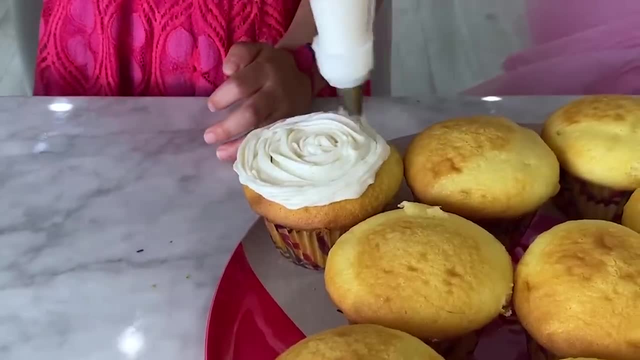 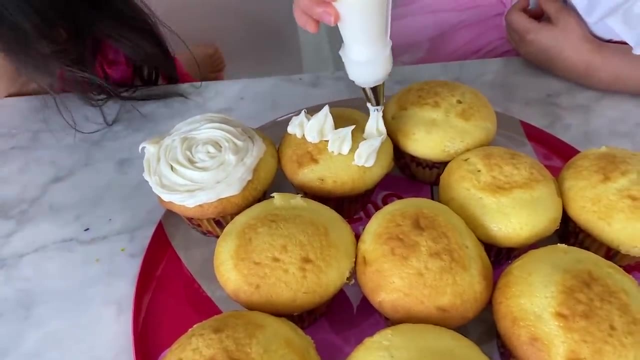 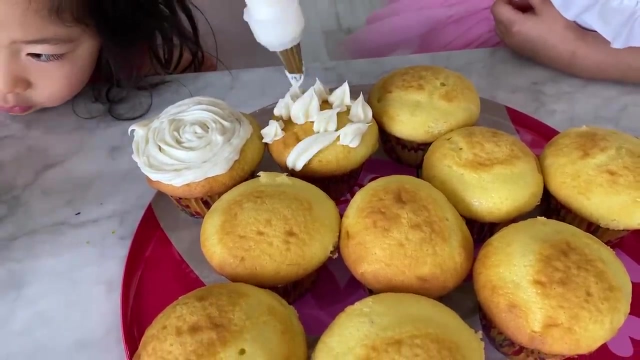 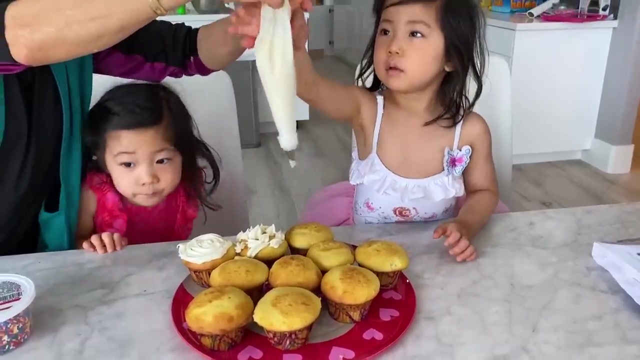 beautiful. you can do like this too. yeah, anything you want, it's the cupcake. you can decorate it any way you like. I want it like this. there you go. yeah, of course I want. I want it like a, I want it like a sprinkle like that. good job, you want to try by yourself? there you go, hi, hi. 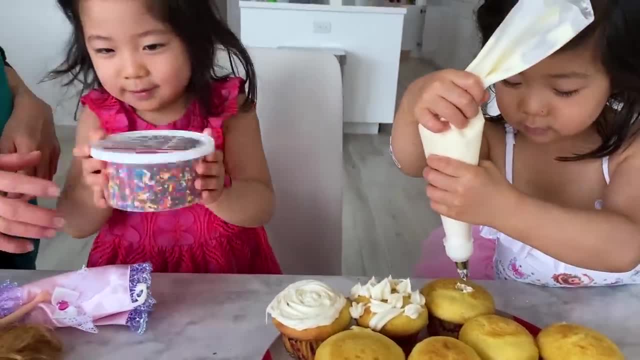 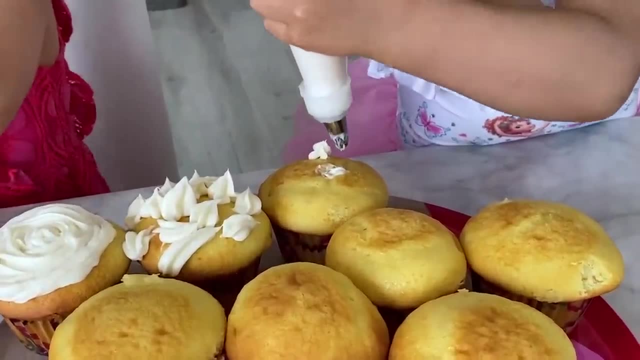 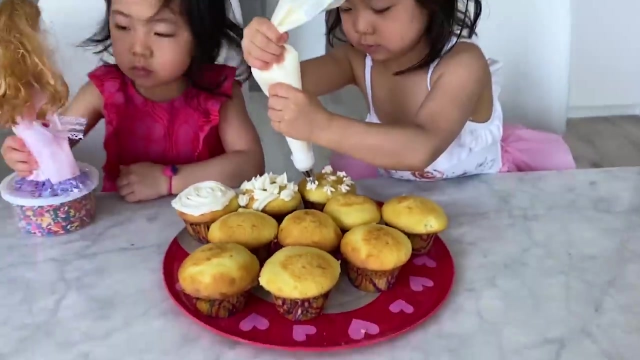 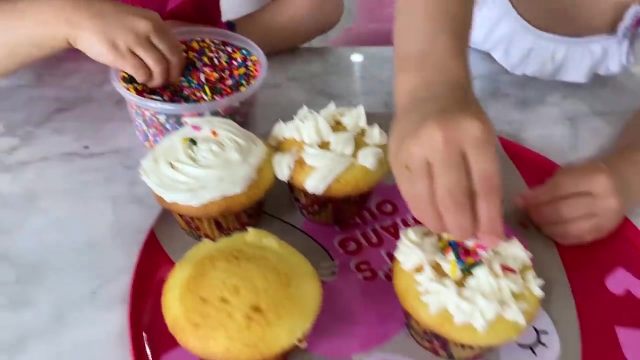 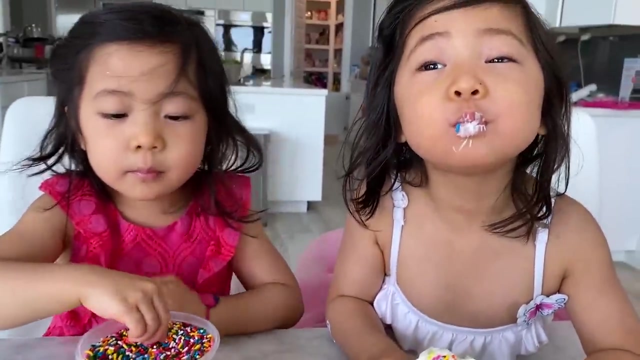 okay. yeah, we can add sprinkle later. okay, there you go. wow, good job. you have to squeeze hard cake squeeze, there you go. wow, okay, so a good job. yeah, so now we're putting sprinkles. good, good job, beautiful good job girls. yeah, you can try, but it's not gonna stick. but you can if you want to.